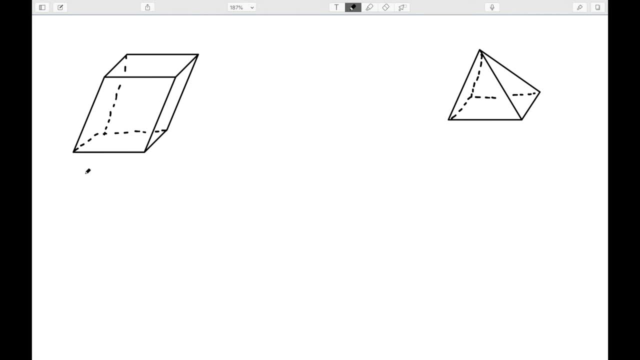 Here I have two polyhedra, So this one has a total of six faces: The front and the back, the left, right and the top and the bottom. It has 12 edges, Which are the straight lines and the dotted lines that you see here. 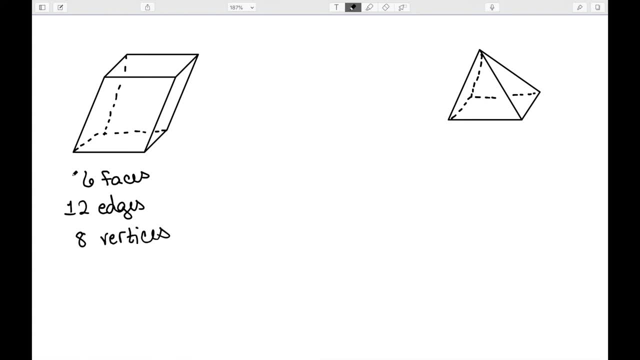 And then a total of eight vertices, Which are the corner points, like this one here Over here. this one has five faces, eight edges and five vertices. On the other hand, if I consider a sphere, this is not a polyhedron. 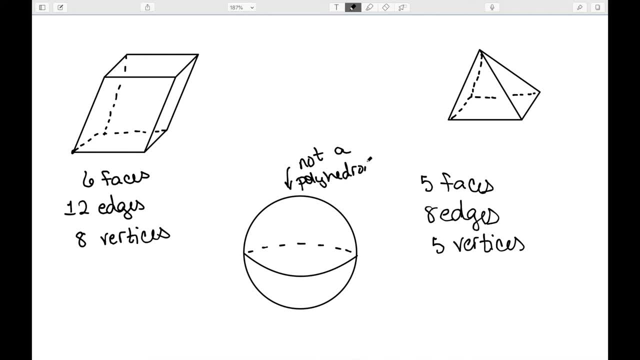 Since it does not have any faces. the outside is not made up of polygons, So a sphere is actually not a polyhedron. I now want to talk about platonic solids. There are five special polyhedra that are completely regular and uniform all around, And these are known as platonic solids, Named after Plato. 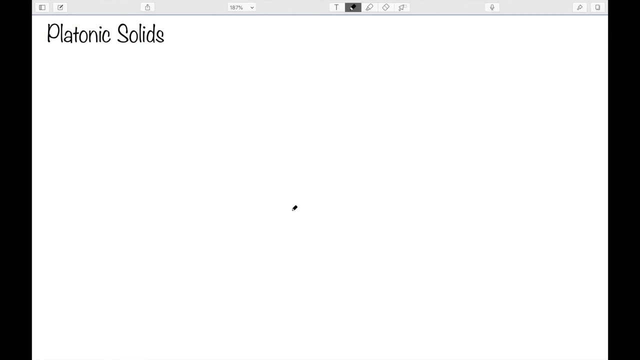 And these are known as platonic solids Named after Plato. And these are known as platonic solids Named after Plato, Who thought these solid shapes associated with earth, fire, water, air and the whole universe. So let's look at each one of the platonic solids individually. 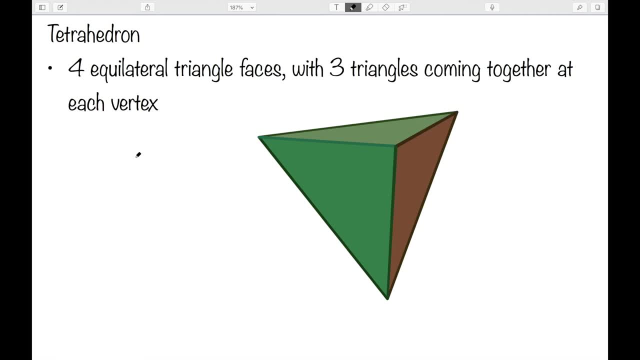 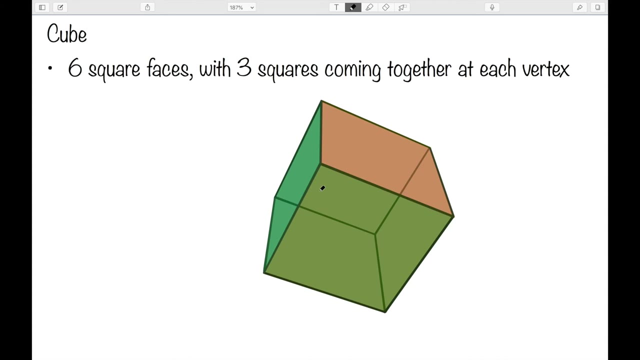 The first platonic solid is a tetrahedron. This has four equilateral triangle faces, with three triangles coming together at each vertex, As we can see in this picture here. Next, we have a cube which is made up of six square faces with three squares. 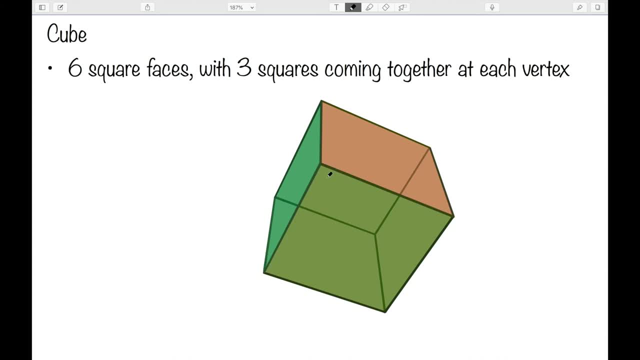 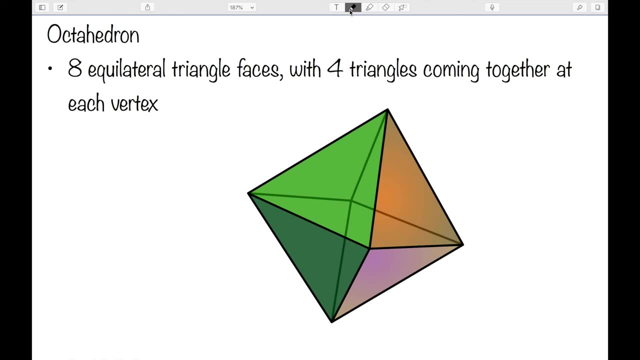 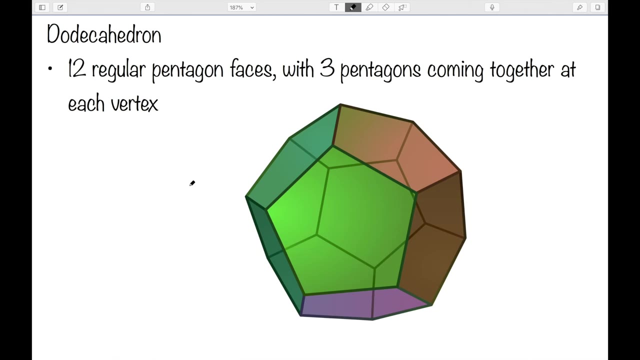 coming together at each vertex. An octahedron which has eight equilateral triangle faces, with four triangles coming together at each vertex. A dodecahedron which has 12 regular pentagon faces, with three pentagons coming together at each vertex. 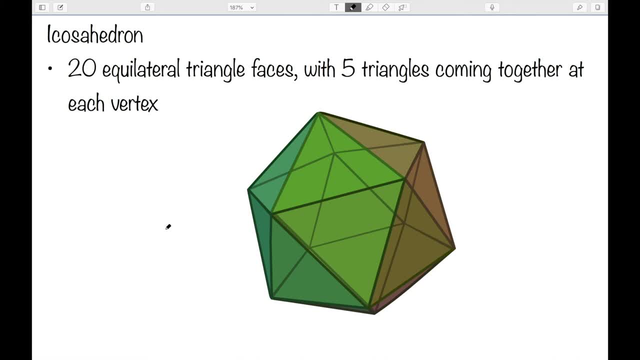 And finally, an icosahedron which has 20 equilateral triangle faces, with five triangles coming together at each vertex. So the names of the platonic solids make sense, because hedron comes from the Greek word for base or seat. Tetra, oca, dodeca and icosa mean 4,, 8,, 12, and 20 respectively. So, for instance,